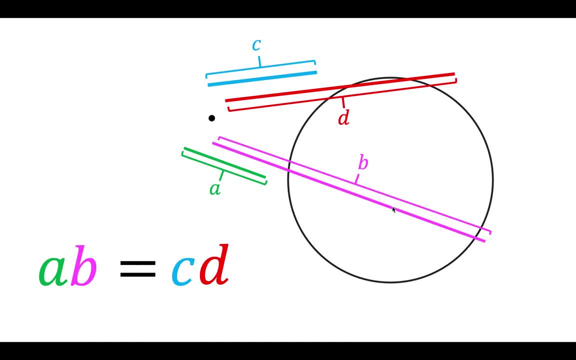 of the entire line. B is the full length of the entire line, So it looks like that Where D and B are the full lengths of the line. Some people think they are just a part inside the circle, but that is a mistake, So be careful. 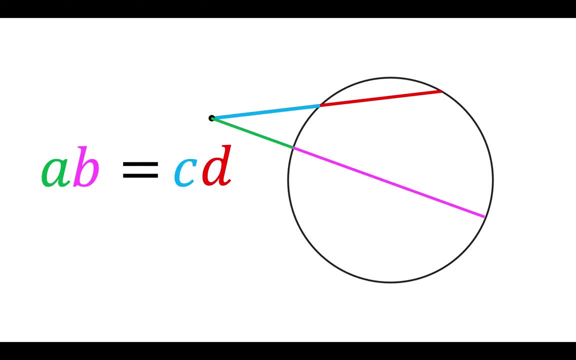 Now we have these two theorems where we're going to use these for an example. So here we know that 4 times a question mark is the same as 2 times a 10. They cross inside, so we use our first theorem. So 4 times a question mark equals 2 times 10.. Like that. So 4x is equal. 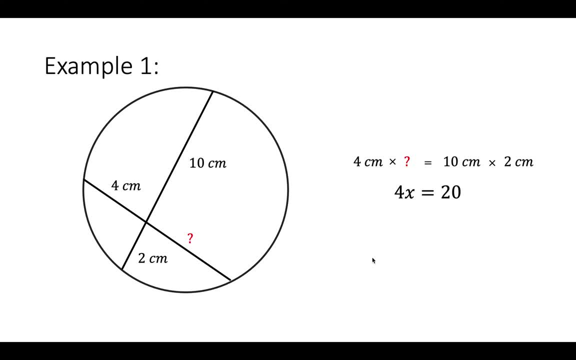 to 20.. We divide by 4 and we get. the missing number is 5 centimetres, Like that, And that's the final answer. Now example 2.. This is where they cross outside of the circle, so we use the second theorem. 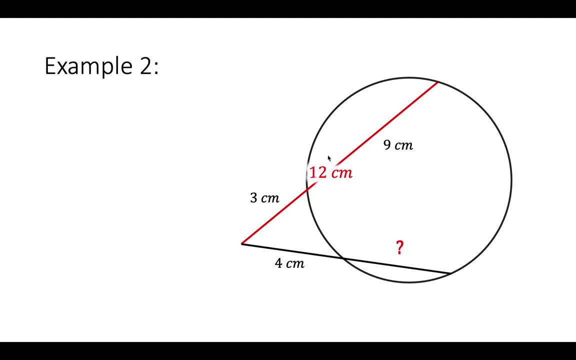 The full length of this line is like this: So we've got the first line, we've got the second line, and then we've got the last line. So we've got the first line and then we've It's 3 plus 9, so be careful. 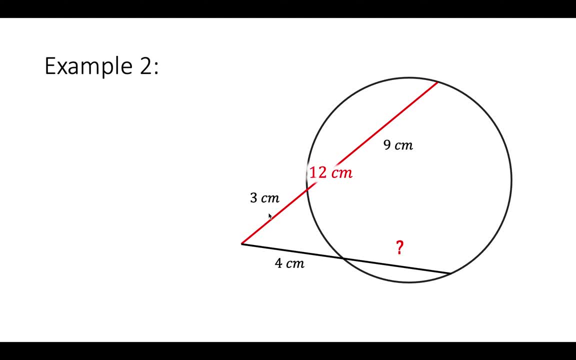 Some people think it's just a 9-year multiply. What we do is use the full length of the red line, So 3 times 12 is equal to 4 times the length of the full line, which will be 4 centimetres, and the question mark together. 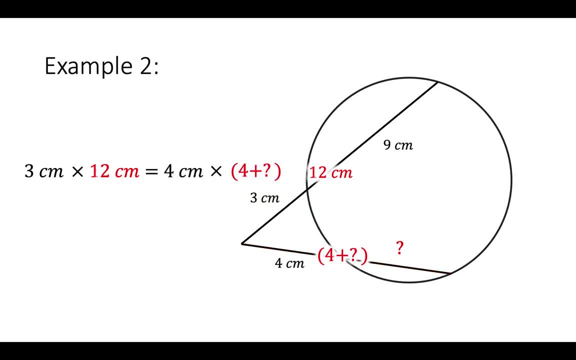 which is 4 plus the question mark, Like that. But 3 times 12 is 36, and it's equal to 4 times 4 plus the question mark. Divide by 4, we've got 9 equals 4 plus the question mark. 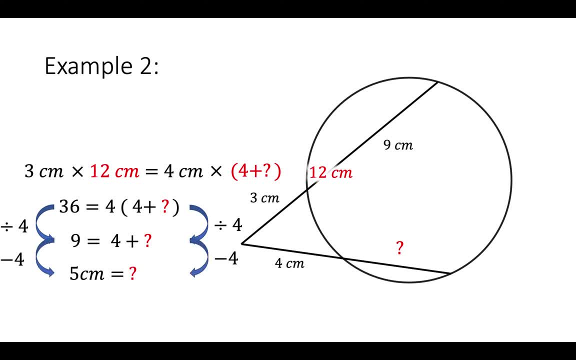 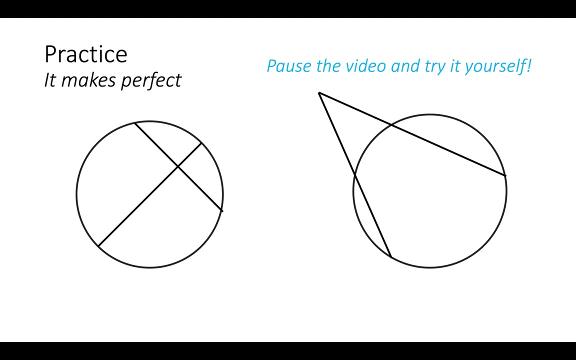 and we find that the question mark is 5 centimetres, Like that. So the final answer is that the missing length from here to here is 5 centimetres. I've got some practice questions for you here where we've got some chords and we've got some lengths. 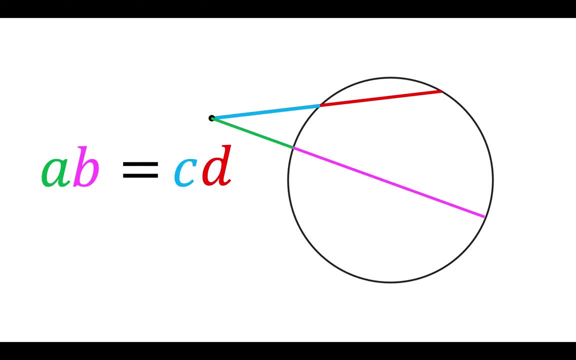 Now we have these two theorems where we're going to use these for an example. So here we know that 4 times a question mark is the same as 2 times a 10. They cross inside, so we use our first theorem. So 4 times a question mark equals 2 times 10.. Like that. So 4x is equal. 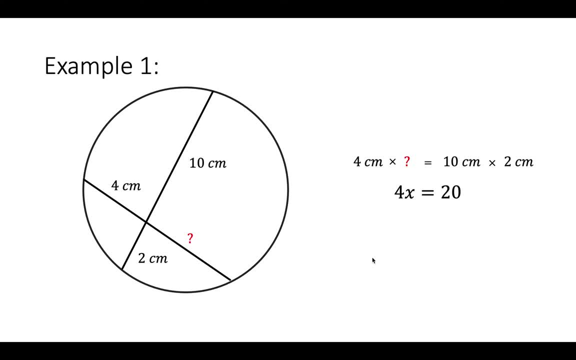 to 20.. We divide by 4 and we get the missing number. it's 5 centimetres, Like that, And that's the final answer. Now example 2.. This is where they cross outside the circle, so we use our second theorem. The full length of this line is where the cross is outside of the circle, so we use the second theorem. This is where the cross is outside of the circle, so we use the second theorem. This is where the cross is outside of the circle, so we use the second theorem. So we've got. 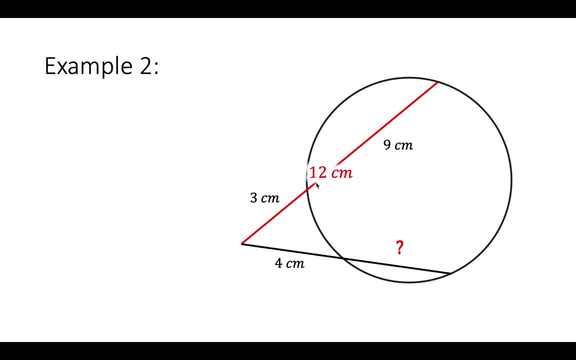 It's 3 plus 9, so be careful. Some people think it's just a 9-year multiply. What we do is use the full length of the red line, So 3 times 12 is equal to 4 times the length of the full line. 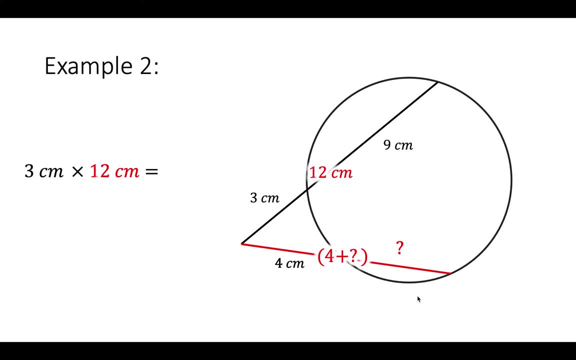 which will be 4 centimetres, and the question mark together, which is 4 plus the question mark, Like that. But 3 times 12 is 36, and it's equal to 4 times 4 plus the question mark. 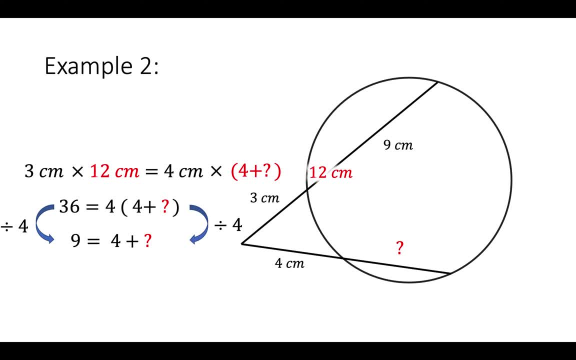 Divide by 4, we've got 9 equals 4 plus the question mark, and we find that the question mark is 5 centimetres, Like that. So the final answer is that the missing length from here to here is 5 centimetres. 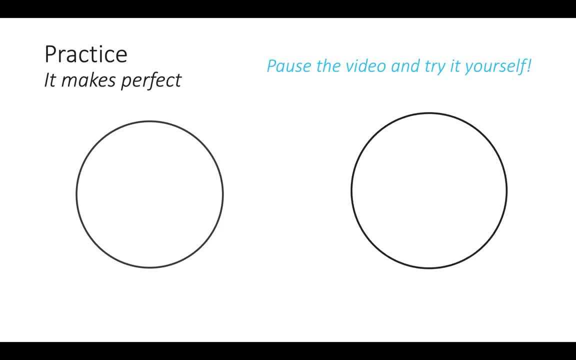 I've got some practice questions for you here where we've got some chords and we've got some lengths. You're trying to find the missing x and you're trying to find the missing a Notice over here that both of these chords are the same length. they are both x.